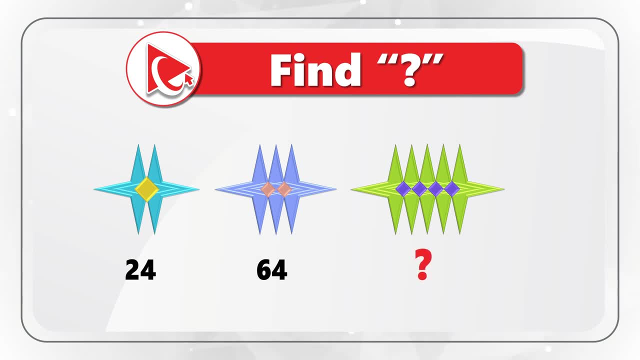 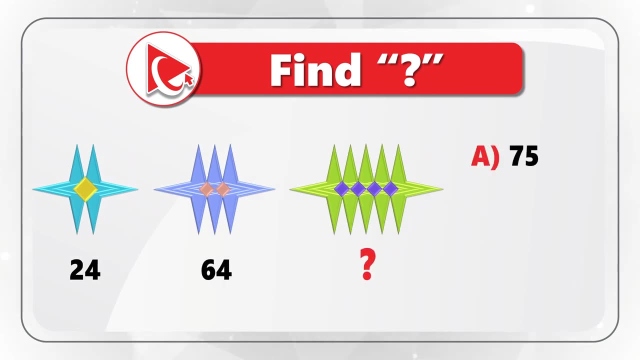 And the third set has a missing number represented by the question mark which you need to calculate and select out of four possible choices: Choice A- 75,, choice B- 96,, choice C 156, and, last but not least, choice D 192. 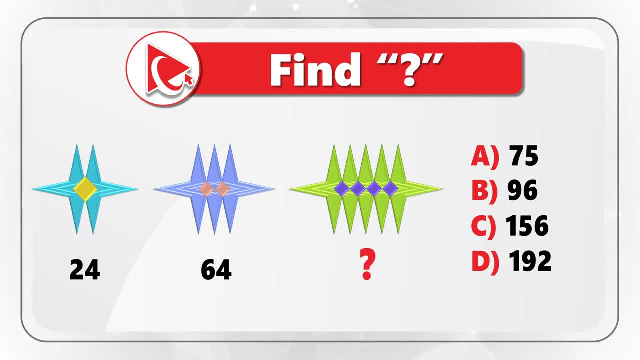 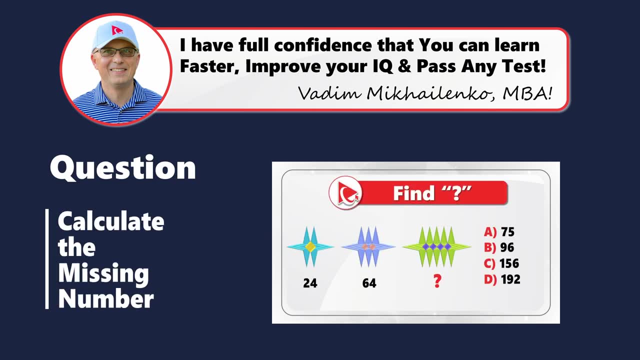 Take a close look to see if you can answer the question. This question is actually very simple and I'm pretty sure you're done by now, So I'm moving forward to share with you my version of the answer And, obviously, if you have a better way to solve it, please make sure to post in comments. 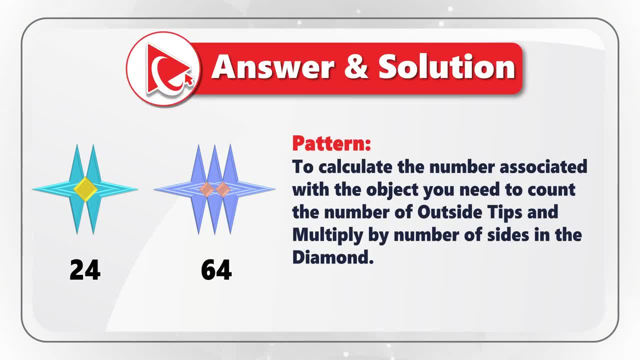 As you might have guessed, the number is calculated based on the number of tips of the stars and number of sides of the diamonds available in each object. Let's look at the example. The first set of blue stars has six tips. Let's count them. 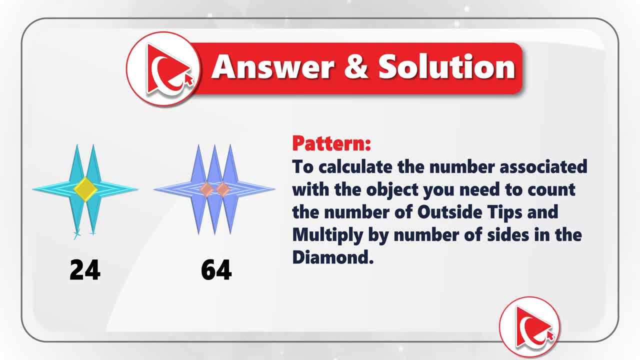 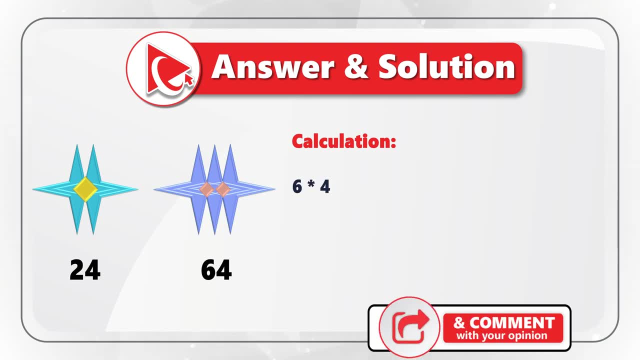 One, two, three, four, five and six, And it only has one diamond which is represented by four sides. Six multiplied by four equals 12.. Can you do the calculations for the second set? I'm here to help you. 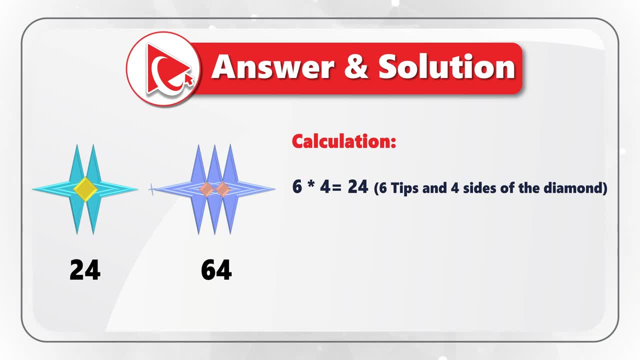 Let's count the tips. We have eight tips on the purple stars: One, two, three, four, five, six, seven and eight. And we have eight sides of the diamonds, because there are two diamonds there. Eight multiplied by eight equals 64.. 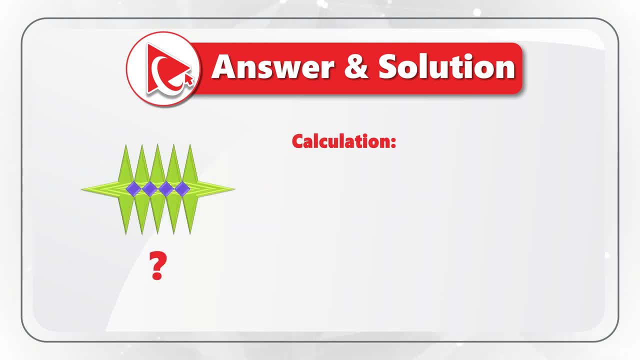 That's how the number was calculated. Let's do the calculations for the missing number. We have 12 tips: One, two, three, four, five, six, seven and eight. Let's count them: Seven, eight, nine, 10,, 11,, 12,, which are represented by 16 sides. 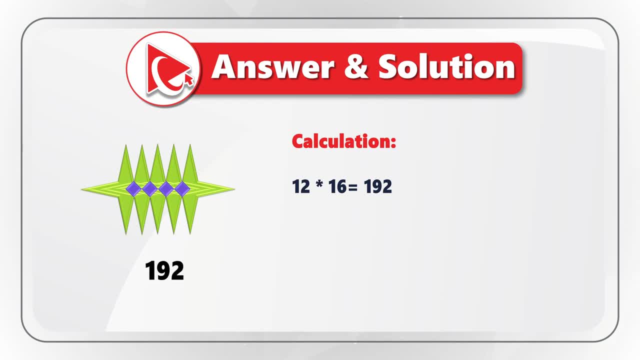 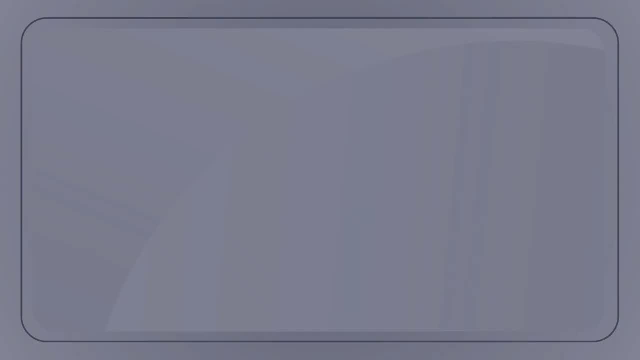 12 multiplied by 16 equals 192,, which is represented by choice D. So the correct answer here is choice D, 192.. Did you get to the same answer? If not, please make sure to post your answer and solution in comments. 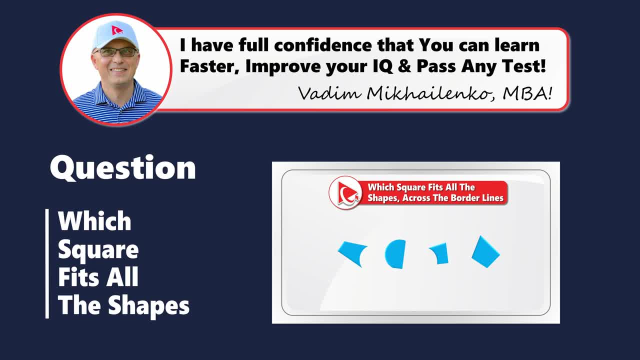 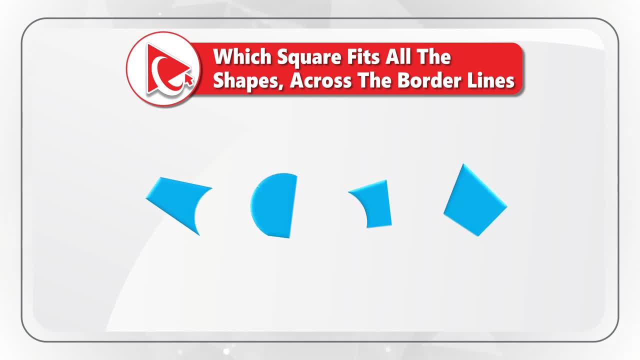 Which was initially designed to test your spatial reasoning, but also could be used to test your cognitive abilities and analytical skills. Okay, Let's move on to the next step. Let's start with four shapes And you need to find the square which fits all the shapes across the borderlines. 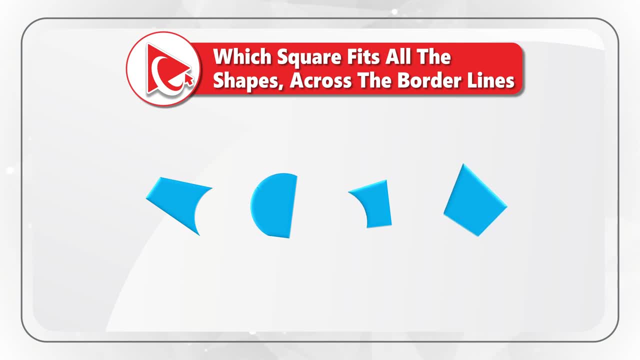 You need to select one square out of four possible choices based on the borderlines. presented Choices are A, B, C and D. Take a close look to see if you can identify the item. Seems challenging, Don't you think so? 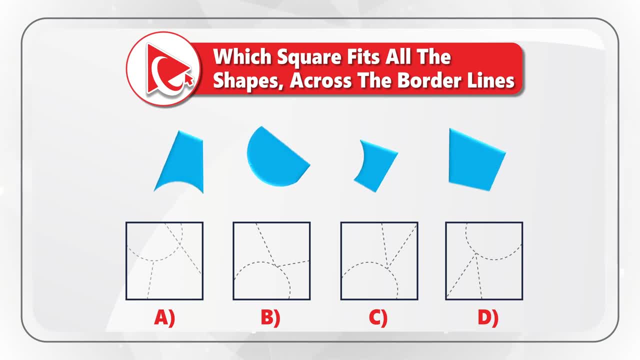 Let me give you a hint. Try to see if you need to rotate the shapes or do any other manipulations with the shapes. Let me give you a hint: Try to see if you need to rotate the shapes or do any other manipulations with the shapes. 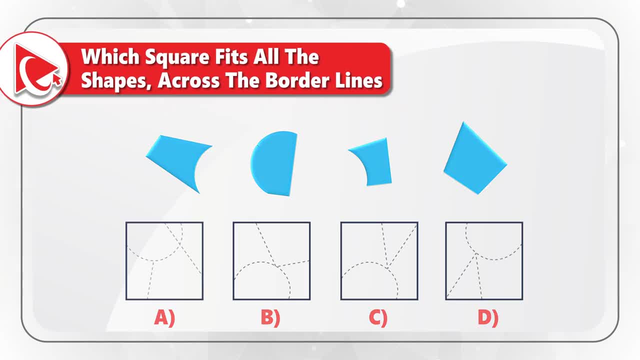 Let me give you a hint: Try to see if you need to rotate the shapes or do any other manipulations with the shapes Before trying to fit them. Are you ready? now Let's move forward and I'll share with you my version of the answer and, obviously, if 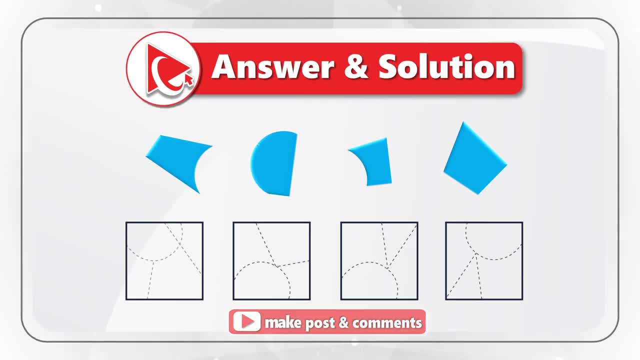 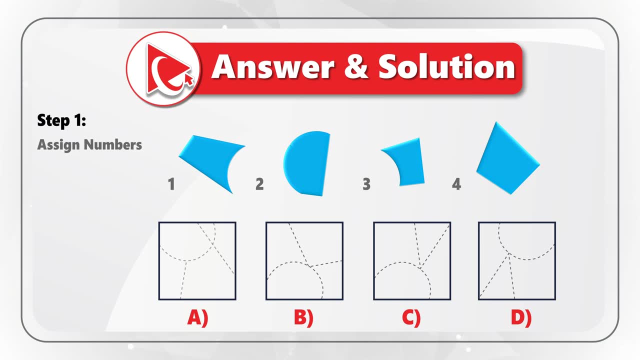 you have a better way to solve it, please make sure to post in comments. But I was able to solve this challenge in three simple steps. Step one: you need to assign the numbers. In step two, you need to rotate the shapes to position them to fit. 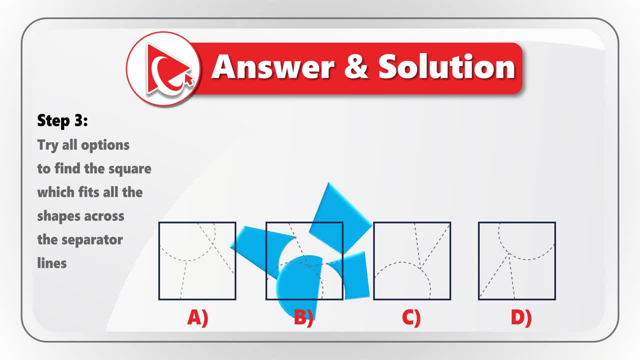 And in the last step, three, you need to try all the options to find the square which fits the shapes across the separator lines. let's look at the example. let's first assign each shape a number, because we have four shapes. the numbers will be 1, 2, 3 and 4.. the second step is the 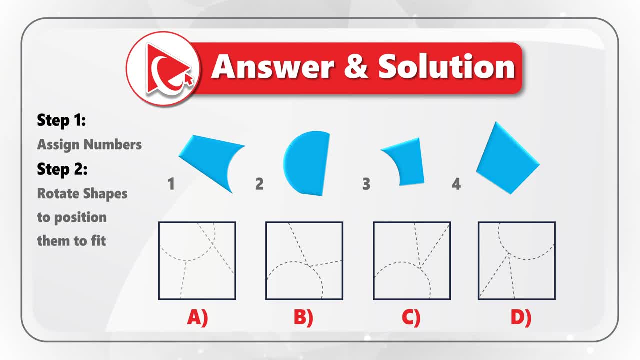 hardest in this step. you need to rotate the shapes to position them to fit and you need to find the closest square which fits all the shapes. let's rotate each shape to get them into the correct position. let's rotate shape 1, now shape 2, now shape 3 and now shape 4.. you need to watch out. 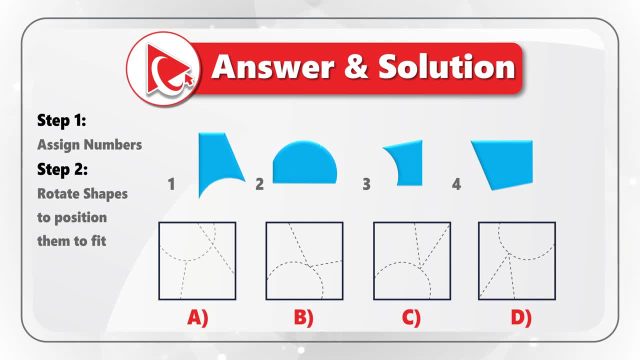 because rotation could be in the different directions, as it happens in this question as well. and once you have all the shapes rotated correctly, we need to move to step 3, where we will try all the options to find the square which fits all the shapes. square a is not going to fit them because 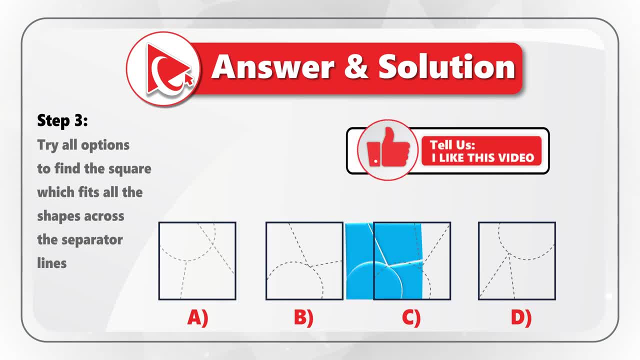 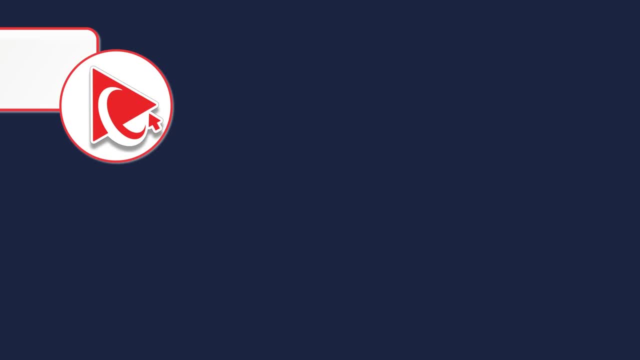 there are five shapes based on the border lines. square c also is not going to fit them. say same with square D. So the only correct answer here is choice B. Did you get to the same conclusion Or maybe you found a better way to solve it? Please make sure to post your answer and rationale. 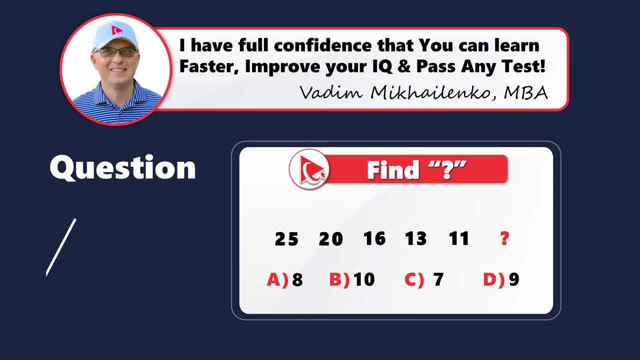 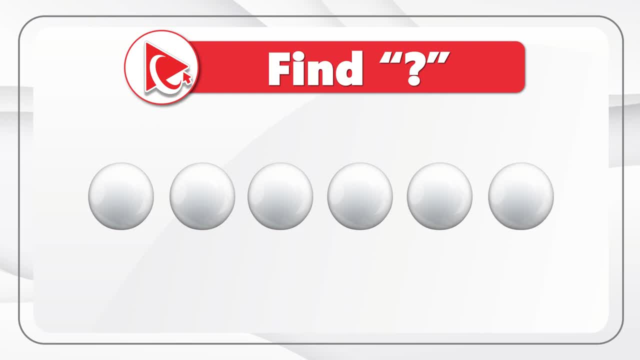 in comments. I enjoy solving pattern questions because they're so easy to understand but sometimes not so easy to solve. We're presented with the sequence of numbers and we need to find the missing number which is the next in the sequence. The numbers are 25,, 20,, 16,, 13,, 11,. 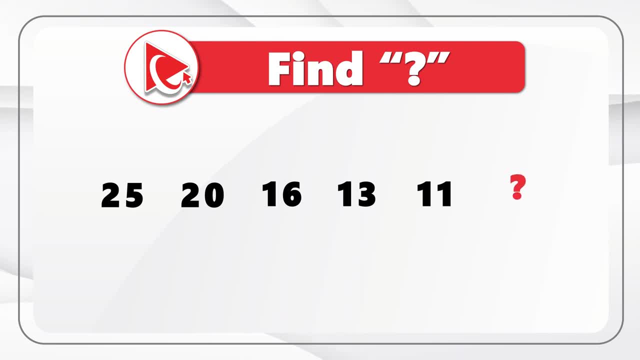 and then comes the missing number. You need to calculate the missing number out of four possible choices: Choices A, B, C and D. Choice A is 8, choice B is 10, choice C is 7, and choice D. 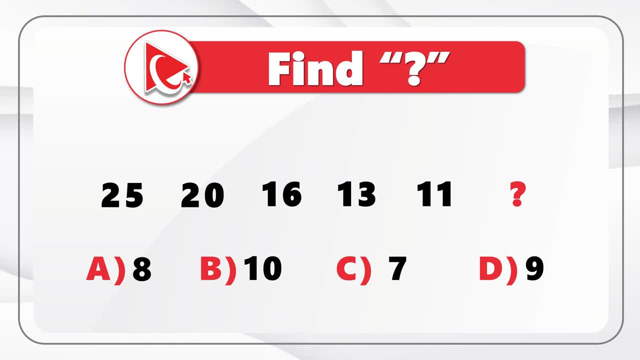 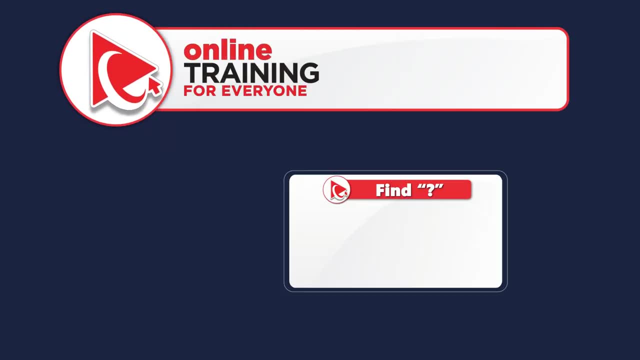 is 9.. Take a close look to see if you can do the calculations and come up with the solution for the missing number. It looks confusing, isn't it? But, believe me, there's a hope at the end of the tunnel, And I'm moving forward to share with you my version of the answer And, obviously, 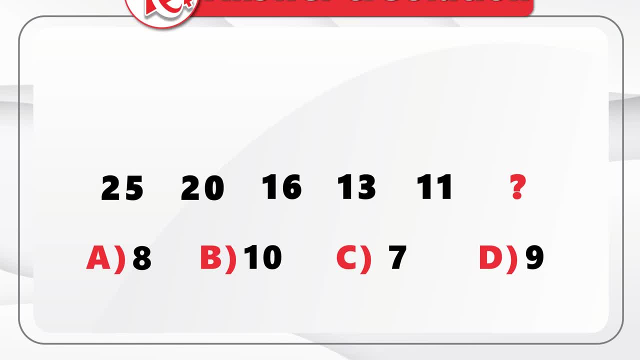 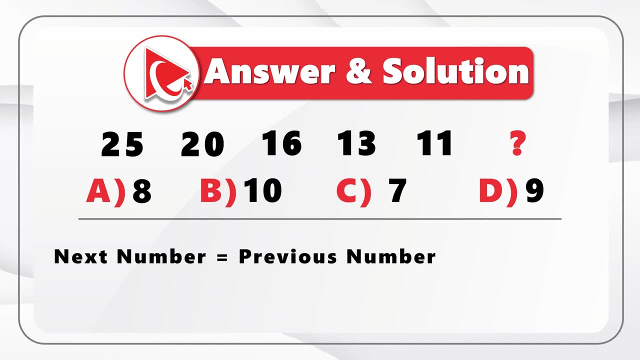 if you have a better way to solve it, please make sure to post in comments. Here we have a concept of decrement, And the pattern is that the next number is calculated as previous number minus decrement, And decrement increases by one with each number in the sequence. 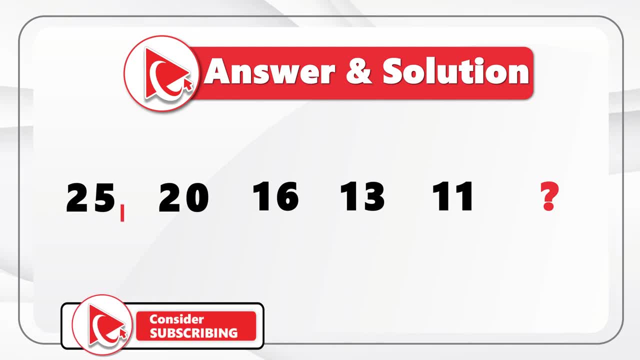 Let's take a close look. Our first number in the sequence is 25.. And our first initial decrement is minus 5.. 25 minus 5 equals 20.. And this is how we come to the second number. Then we decrement the next number And we have a concept of decrement And the pattern is that the next 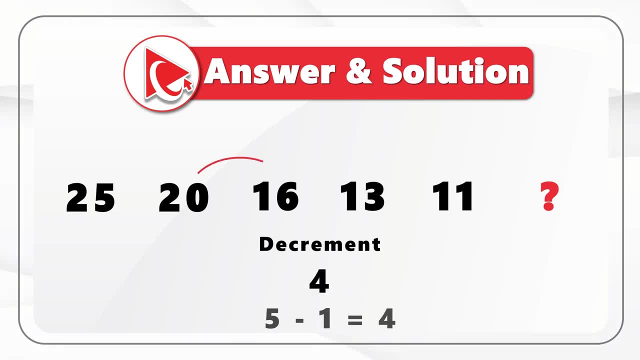 number decreases by one And the decrement becomes minus 4.. 20 minus 4 equals 16.. 16 minus 3 equals 13.. 13 minus 2 equals 11. And 11 minus 1 equals 10.. So the correct answer here is choice B, 10.. 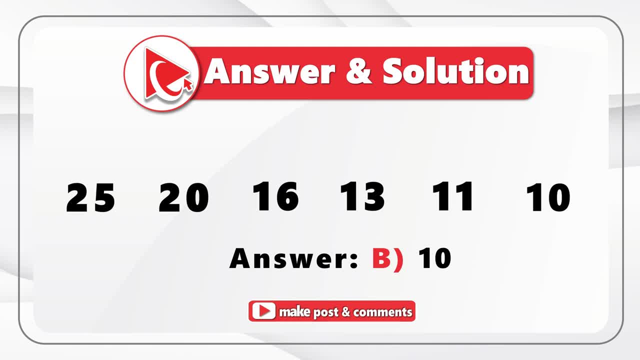 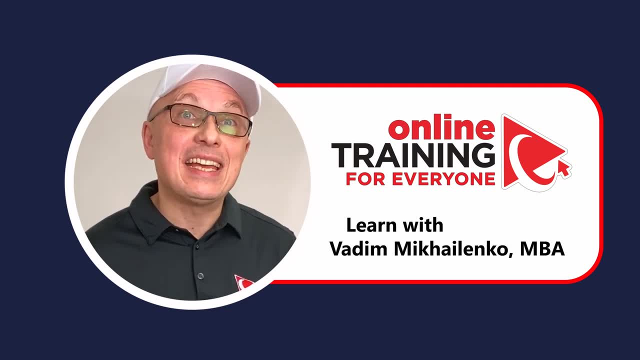 Was your answer different. Please make sure to post your answer and solution in comments then, so we can all learn. Thanks for watching. If the content was helpful, please give us a like and consider subscribing. This is the way for you to tell us that you need more content like this, And we'll make sure to. 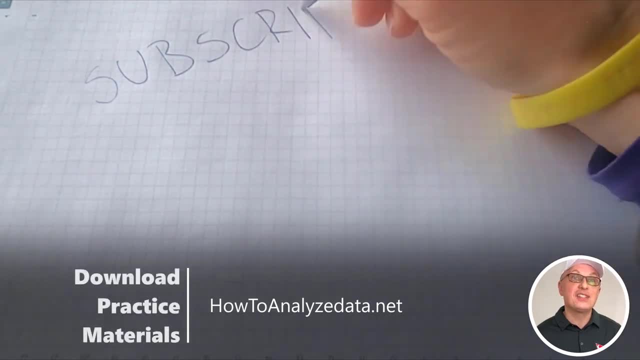 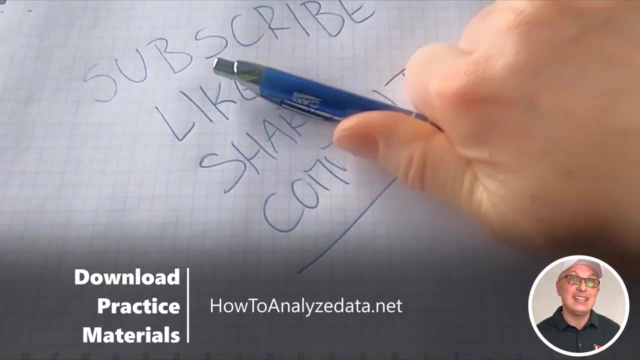 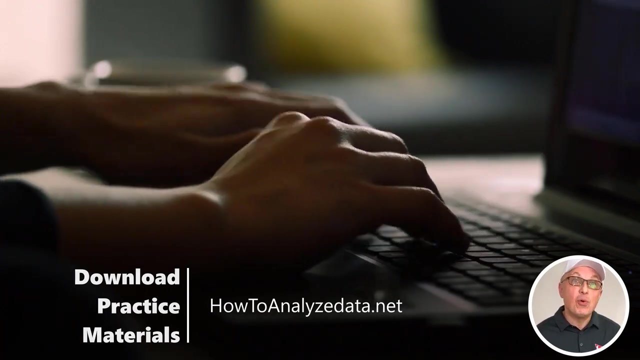 deliver it for you in the future. For links and resources referenced in this video, please check the description. You can also go directly to our website howtoanalyzedatanet to find what you're looking for and download the materials. We really thank you for your endorsement, support and.